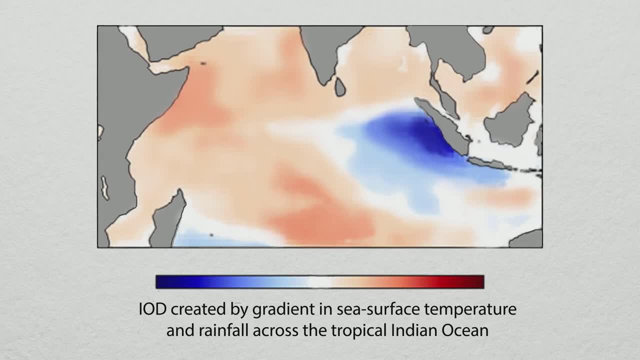 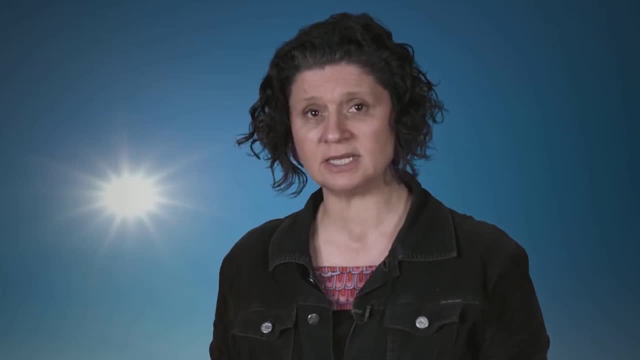 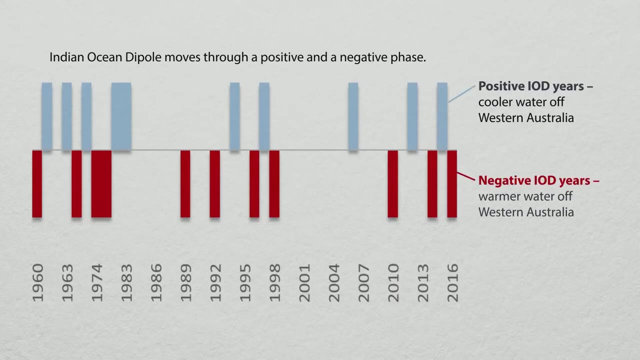 The Indian Ocean Dipole is created by a gradient in sea surface temperature and rainfall along the equator, across the tropical Indian Ocean And, just like El Niño, that gradient shows a seesaw pattern and changes from year to year. The Indian Ocean Dipole moves through a positive and negative phase. 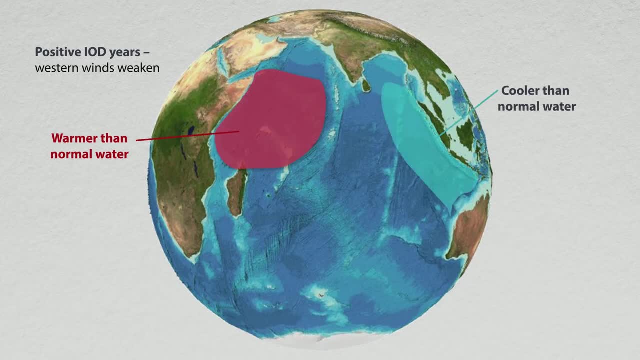 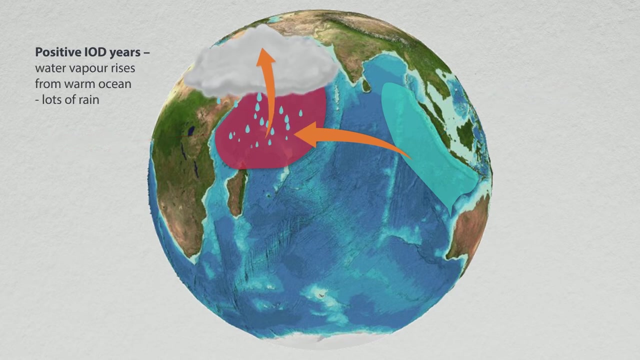 During a positive phase, warmer sea surface water is pushed towards the western Indian Ocean across to the east coast of Africa. The easterly winds and warm water carry lots of humidity, So this increases the rainfall and potentially flooding Over on that part of the Indian Ocean. 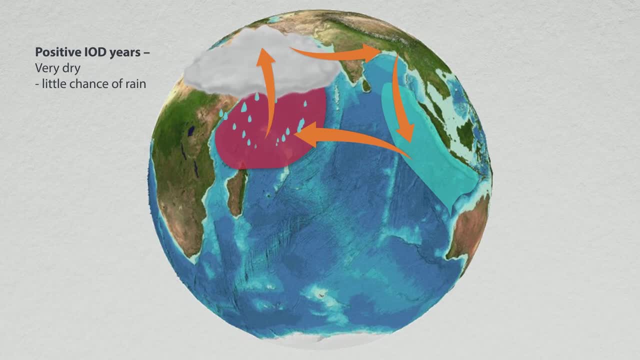 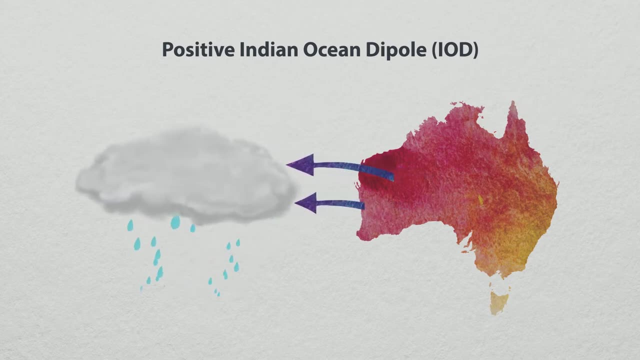 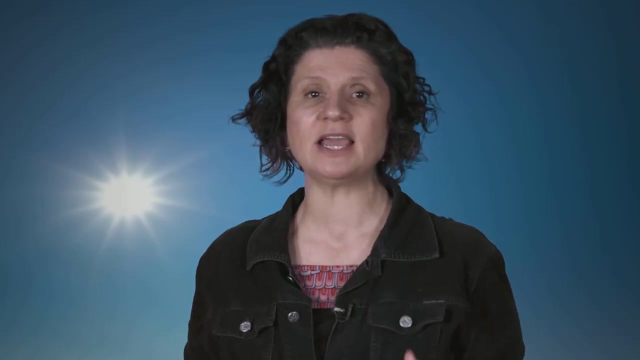 The colder waters around Indonesia and northwest coast of Australia will result in less cloud cover and less rainfall for southern Australia and our Top End. These dry conditions also increase the risk of bushfire in Australia, But in the negative phase of the Indian Ocean Dipole there's the opposite effect. 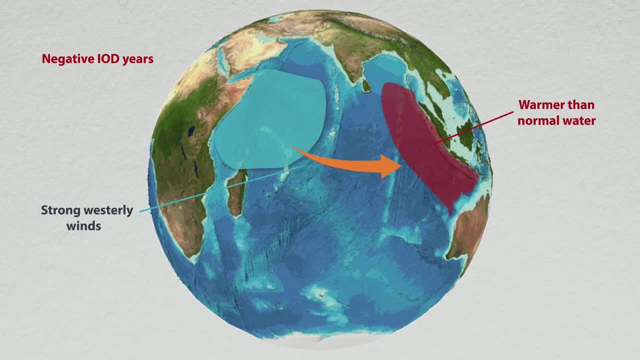 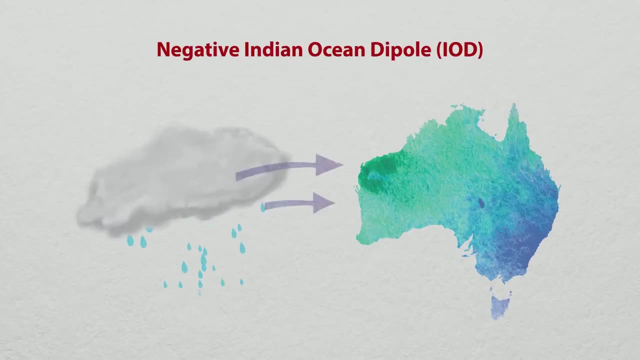 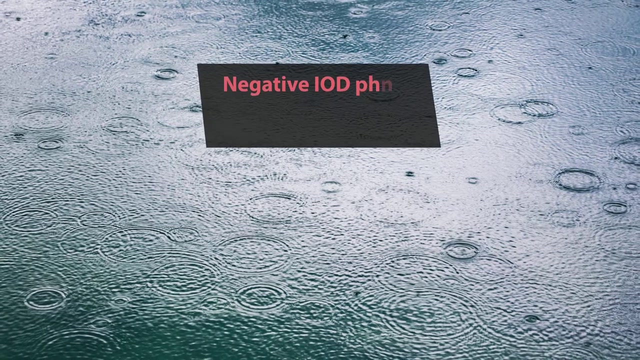 Strong westerly winds push large volumes of warm water towards the west coast of Australia, So now we have higher rainfall. The negative phase of the Indian Ocean Dipole is the one that's really good for us, as it brings more rain, But unfortunately it's a much rarer event and its impact is much more benign. 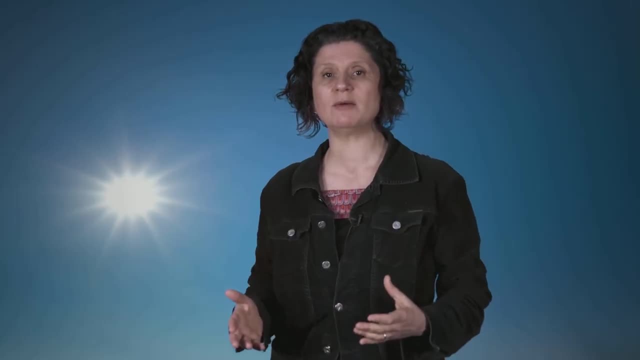 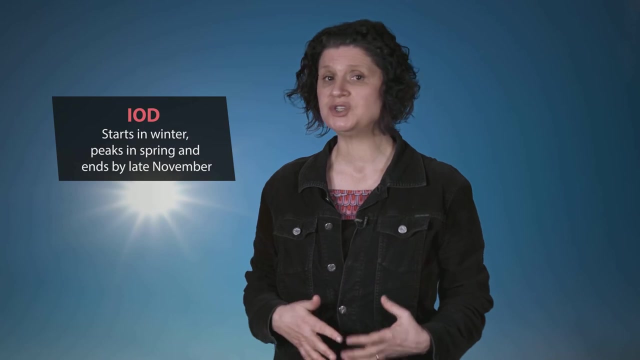 There's not that much more rain. The Indian Ocean Dipole develops earlier in the year than El Niño. It starts in winter and peaks in spring, And usually it's all over by late November. Now that's because the monsoons in East Asia interrupt its cycle. 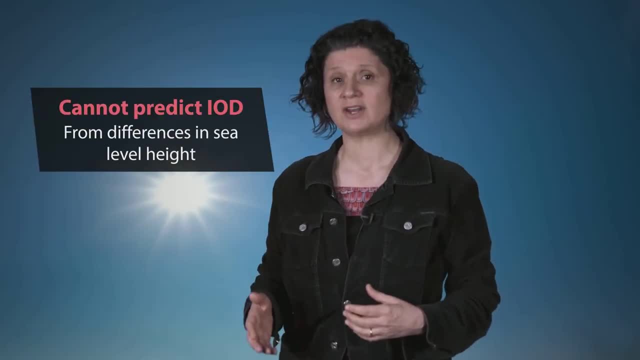 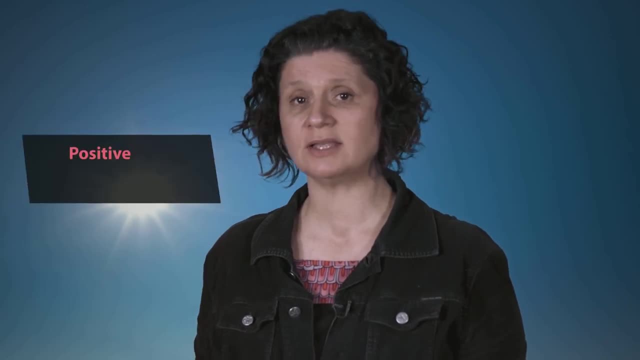 And unfortunately the Indian Ocean Dipole is even harder to predict than El Niño. With climate warming, it's predicted that positive Indian Ocean Dipole events are likely to occur three times more often than they have in the past- Unlucky for us. 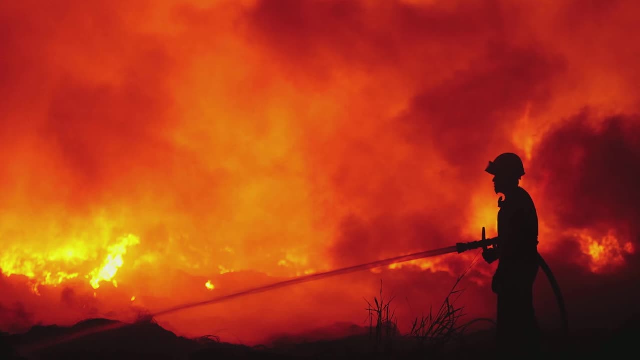 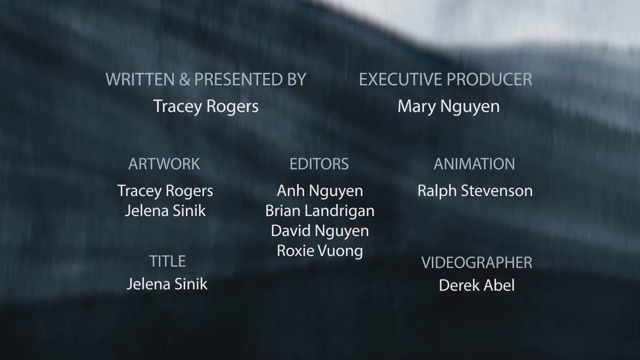